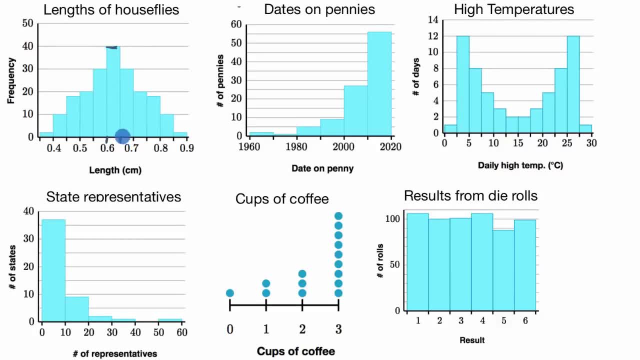 Looks like there's about 40 houseflies there, And then if you say between 6 1⁄2 and 7: 1⁄10,, there's about 30 houseflies, And if you were to say between 5 1⁄2 1⁄10 and 6: 1⁄10,. 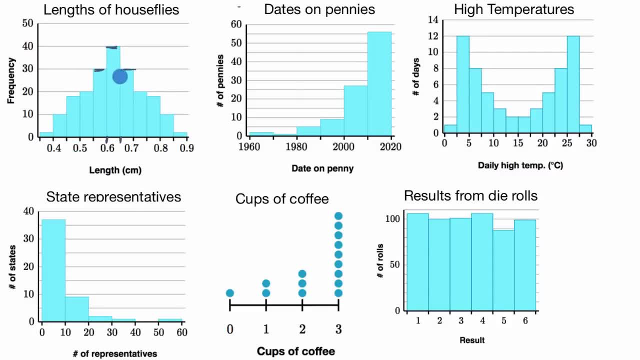 it looks like it's about the same amount. This type of distribution is usually described as being symmetric. Why is it called that? Because if you were to draw a line down the middle of this distribution, both sides look like mirror images of each other. 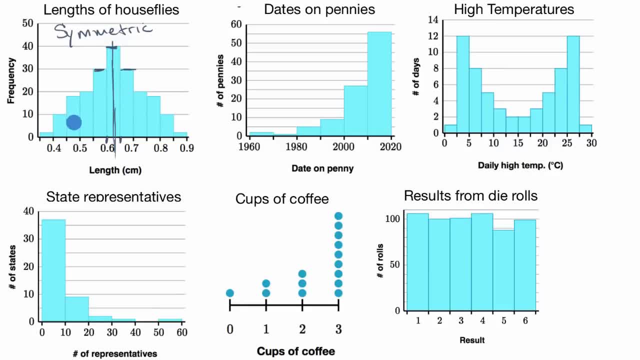 This one looks pretty exactly symmetric, but more typically, when you're collecting data, you'll see roughly symmetric distributions. Now here we have a distribution that gives us the dates on pennies. So someone went out there observed a bunch of pennies. 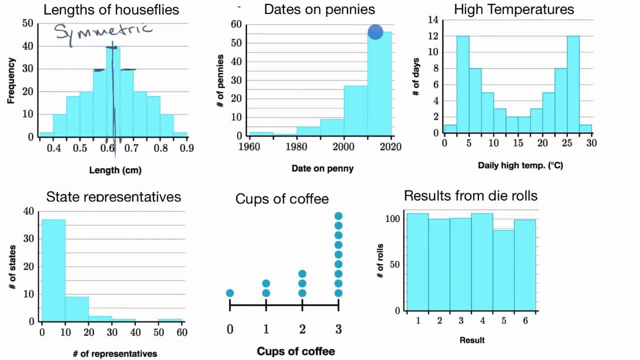 looked at the dates on them, They saw many pennies looks like a little bit more than 55 pennies had a date between 2010 and 2020, while very few pennies had a date older than 1980 on them. 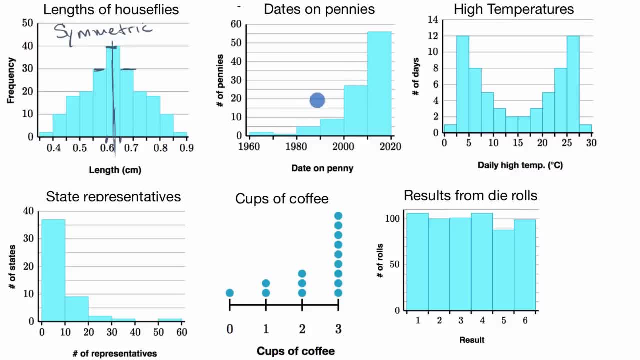 And this type of distribution: when you have a tail to the left- you can see it right over here- you have a long tail to the left. This is known as a left skewed distribution- Left skewed. Now, in future videos, we'll come up with more technical definitions. 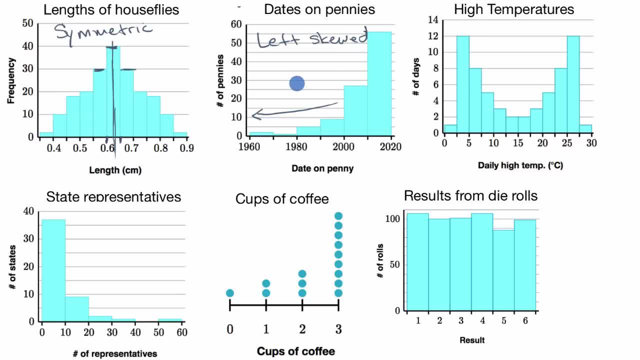 of what makes it left skewed. But the way that you can recognize it is you have the high points of your distribution on the right, but then you have this long tail that skews it to the left. Now the other side of a left skewed. 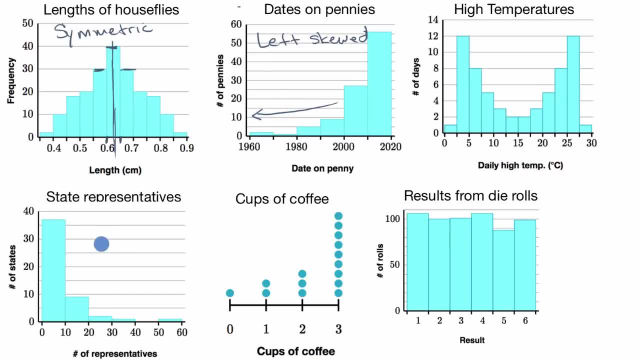 you might say: well, that would be a right, skewed distribution, And that's exactly what we see right now. This is a distribution of state representatives And, as you can see, most of the states in the United States have between zero and 10 representatives. 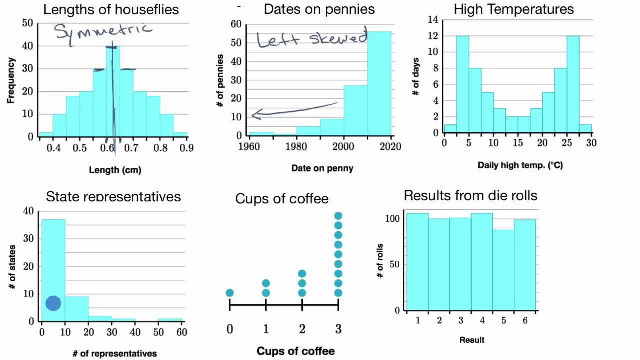 It looks like it's a little over 35.. None of them actually have zero. They all have at least one representative, but they would fall into this bucket, while very few have more than 50 representatives. So here where the bulk of our distribution is to the left. 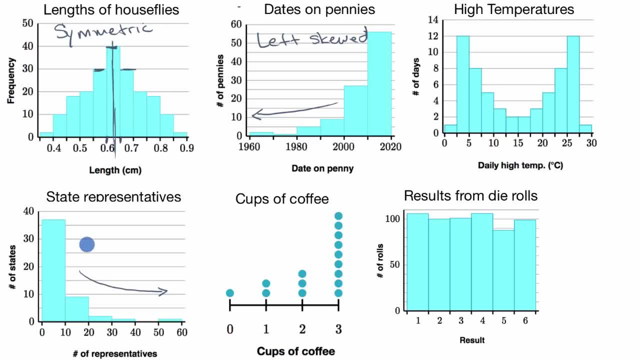 but we have this tail that skews us to the right. this is known as a right skewed distribution- Distribution. Now, if we look at this next distribution, what would this be? Pause this video and think about it. Well, this could be a distribution.